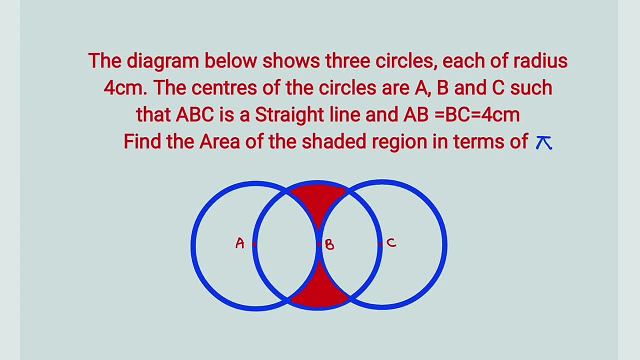 Hello, good day viewers. Here is another nice geometry question. The question reads: the diagram below shows three cycles. you can see them- A, B and C, each of radius 4 centimeters. The centers of the cycles are A, B and C, such that A- B- C is a straight line and A- B is equal to. 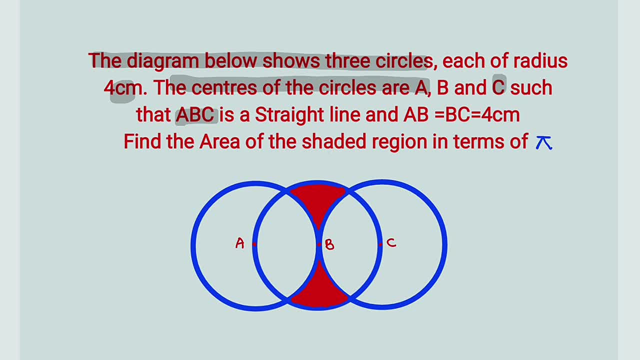 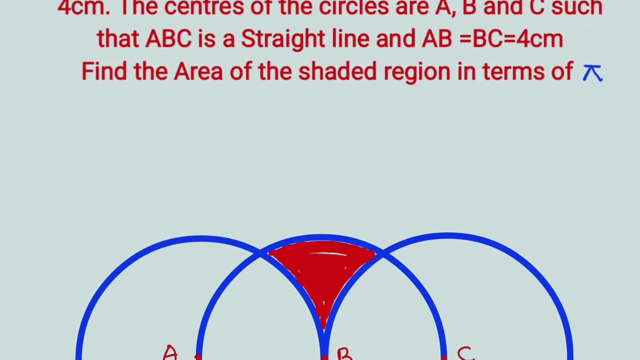 B, C equal to 4 centimeters. We are asked to find the area of the shaded region marked red. All right, let's get started with the solution And we want to leave our answer in times of pi. Let us make some sketch here. From the question, we have learned that A, B, C is a straight line. 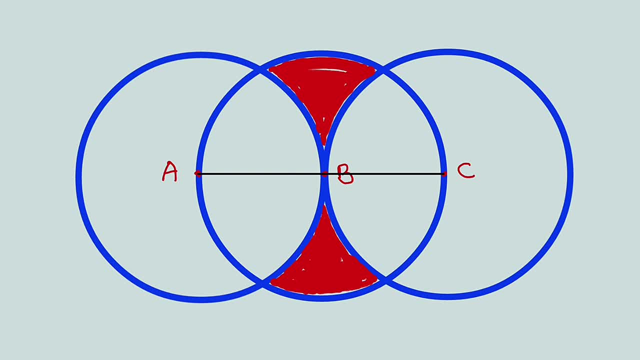 So let's connect A, B and C together. And we have also learned that all of these three circles have equal radius, which is 4 centimeters. So we have 4 centimeters here. This is equally 4 centimeters. So I want us to concentrate on this semicircle to the top. We use it to find the value of the. 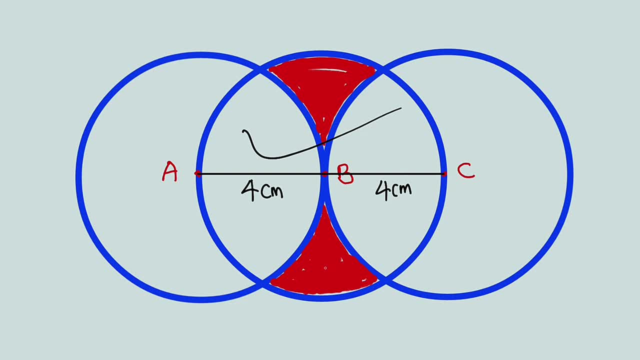 area of this red region, Then we multiply by 2 to obtain the two red regions. All right, let us use the middle cycle. From the center to any part of the circumference is a radius, So this is a radius. This is also a radius, And we have just formed a sector. 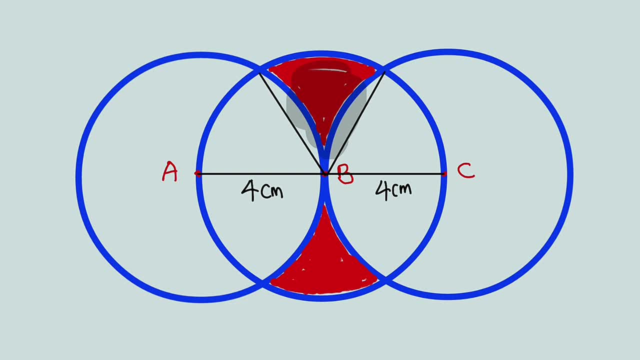 Look at it here. This is a sector And we can use it to find the area of this red region. But how can we do that? We can do that by finding the area of the sector itself. Then we subtract this mini segment. You can see them, two of them. All right, let's go ahead and find the area of that. 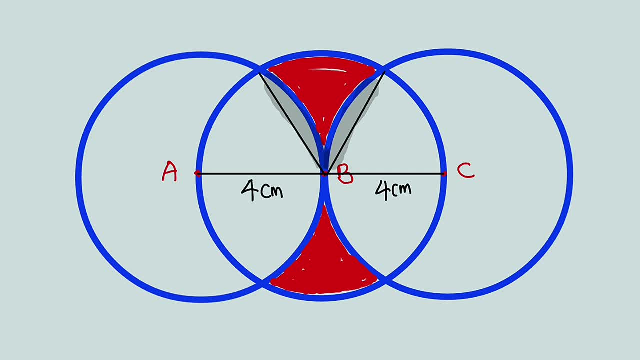 sector first. But also remember that a straight line has an angle of 180.. But observe to the top. we have identical sectors 1,, 2, and 3.. Therefore, if you should divide 180 by 3, you're going to. 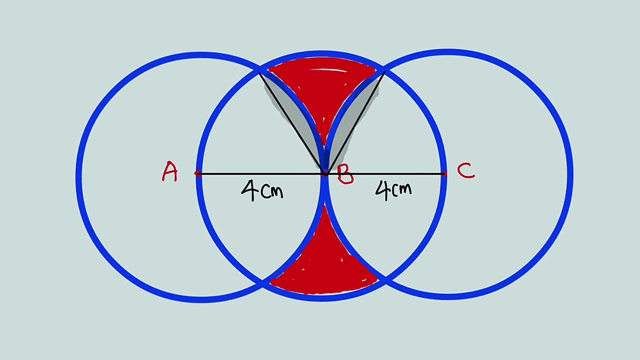 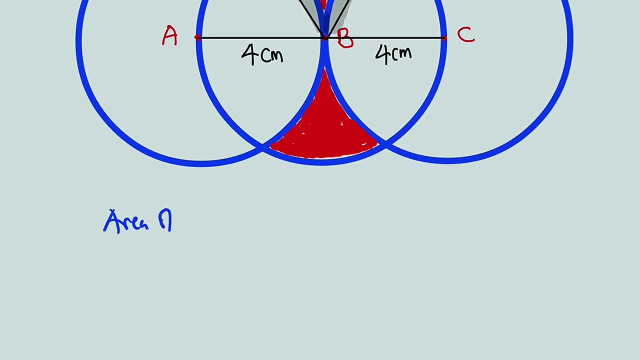 obtain 60 degrees each. Therefore, this sector to the top sustains an angle of 60 degrees. So therefore, the area of a sector will be equal to the angle subtended by that sector out of 360 degrees, multiplied by the area of a cycle which is pi- r squared. 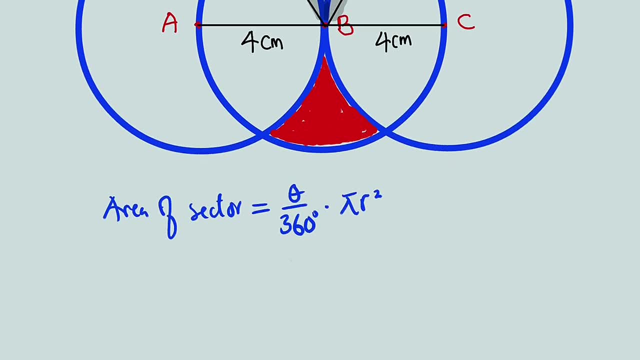 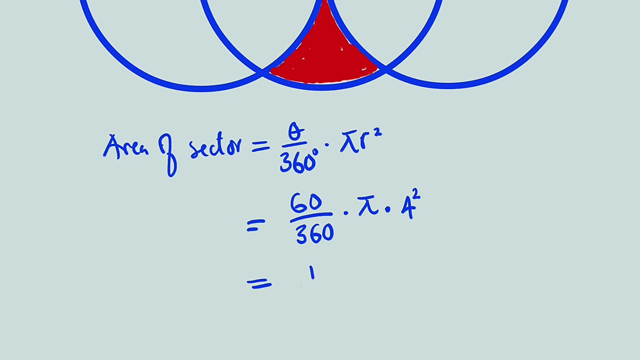 So let's substitute the angles of 10, that is 60 degrees divided by 360 degrees. They multiply by pi, They multiply by r, which is 4 squared. You know, 60 can go into 366 times, right? So this becomes 1 over 6, multiplied by pi, multiplied by. 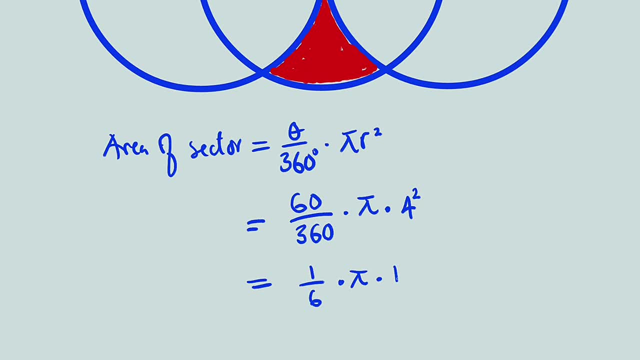 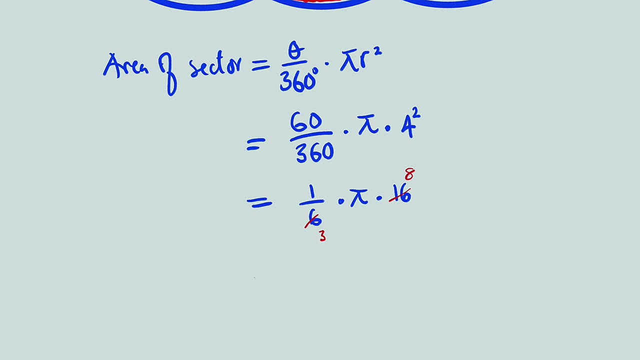 4 squared is 16.. Let's perform a cancellation here. 2 can go into 6 three times and 2 can go into 16 eight times. So we have 8 pi over 3 as the area of the sector. So this is equal to 8 pi over 3. 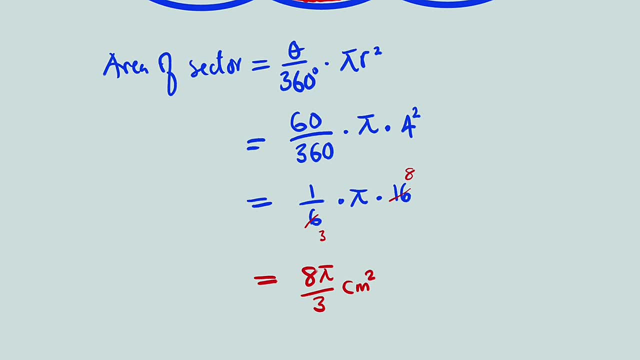 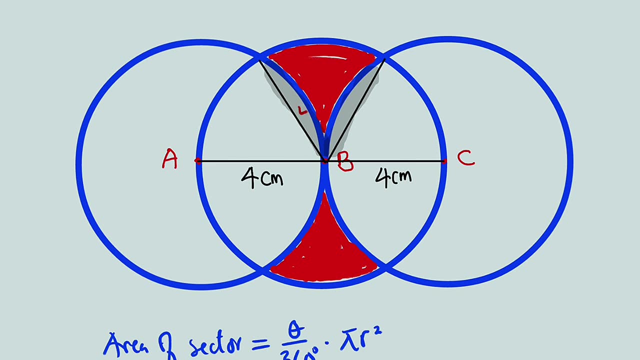 centimeter squared. So this is just the area of a sector. All right, let's come back here. How can we find the area of this segment? Let us find the area of one segment that we multiply by 2 to obtain the area of the two segments. Observe that we can form a triangle right here, which is: 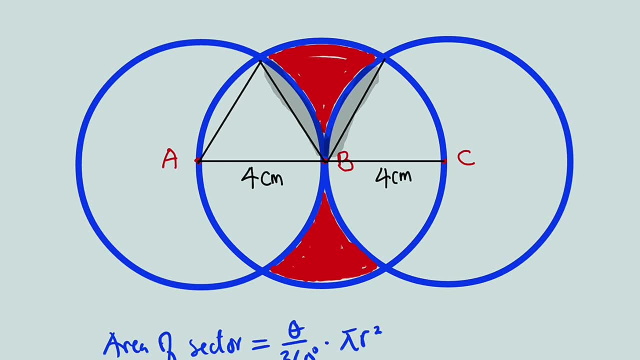 an equilateral triangle with equal size, 4 centimeters each. So if we should find the area of this triangle, subtract it from the area of a sector, because observe that we have a triangle here as well. This is a sector, If we should remove an area of a triangle from an area of a sector. 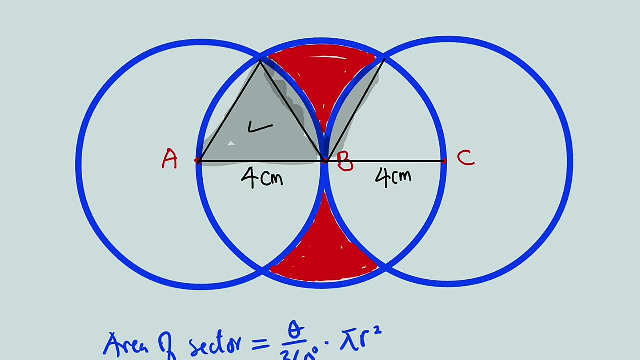 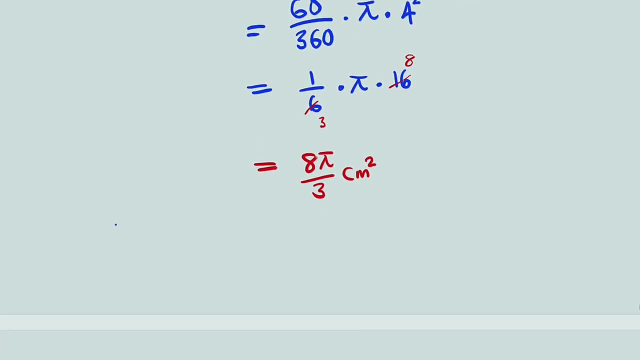 we'll end up getting the area of this segment. So let's go ahead and find the area of this triangle. So area of triangle, Because it is an equilateral triangle, we can use this formula: root 3 over 4.. So the area of a sector is equal to A squared. But since we are dealing with radius here, we can: 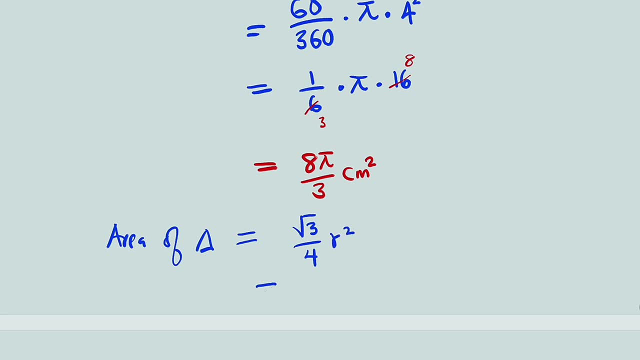 use r. squared is the same thing. A stands for the size of the equilateral triangle, which is equal to root 3 over 4, 4 squared, And this will give us just 4 root 3, because this 4 will cancel 1, 4 here. 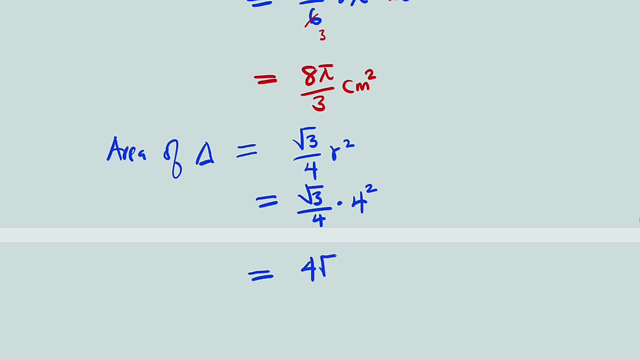 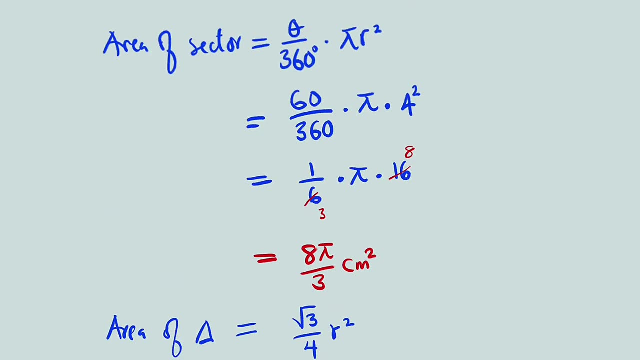 We are left with root 3 multiplied by 4. which is four root three, and this is the area of the triangle. then we need to subtract it from the area of sector, and all of these sectors are identical, so we can use this area right here. 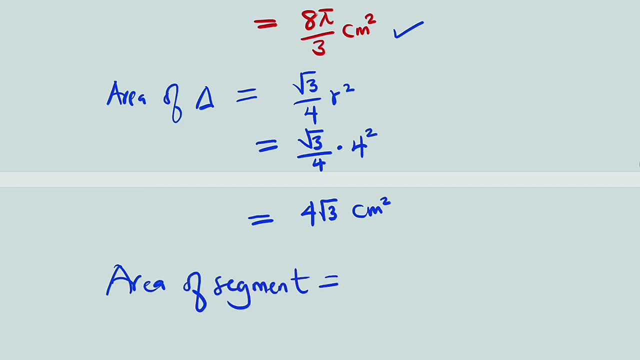 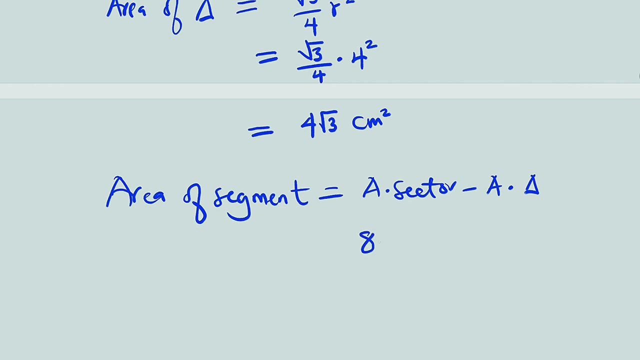 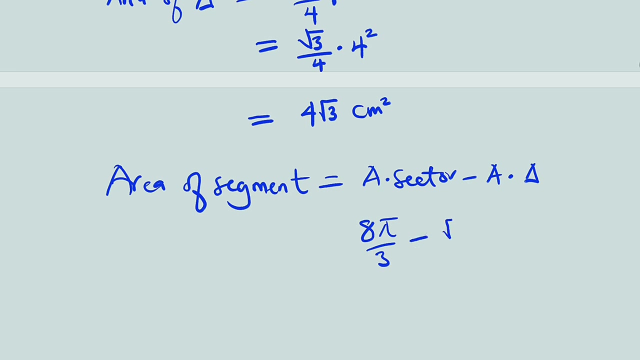 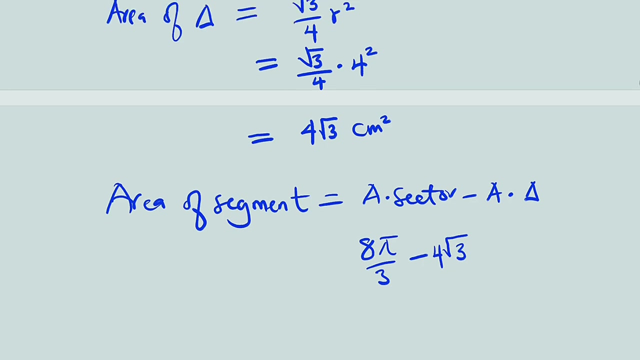 area of segment, it will be equal to area of sector minus area of triangle, and area of sector is eight pi over three, eight pi over three. then we subtract the area of triangle, area of triangle, which is four root three, and this is said to be the area of that segment. but remember, we have two. 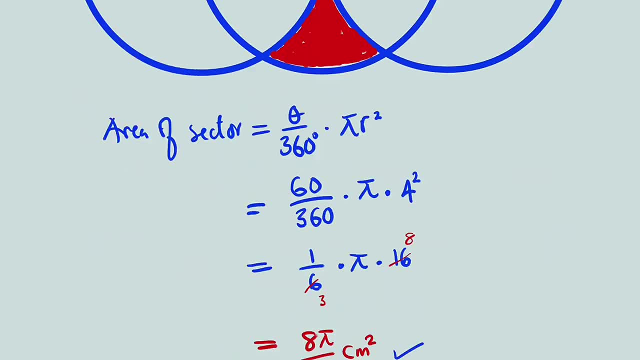 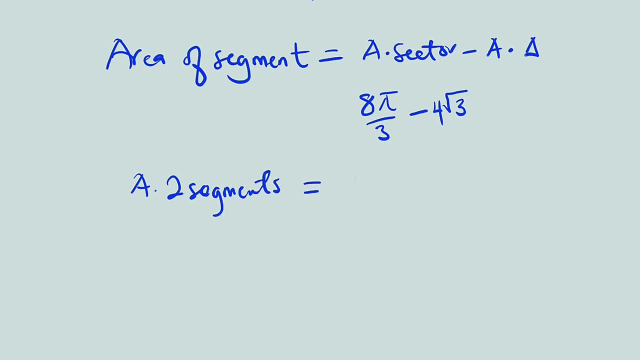 of them. so let's make sure that we have two of them. so let's make sure that we have two of them. multiply by 2.. So the area of two segments is equal to 2 multiplied by 8 pi over 30 minus 4. 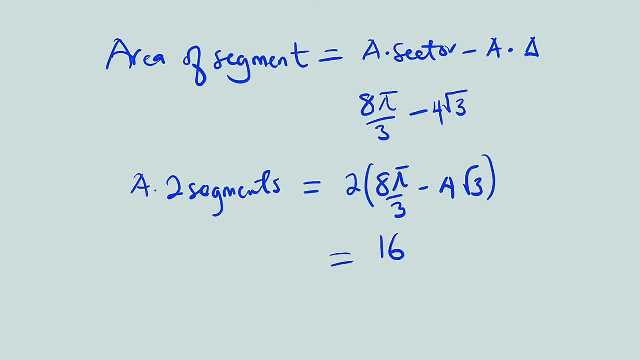 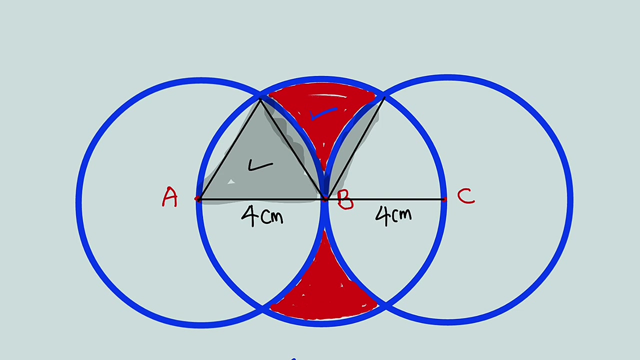 root 30. This will give us 16 pi over 30 minus 8 root 30.. All right, this is the area of these two segments, But remember, we are looking for the area of this red region. Therefore, to find the area of this red region, we can remove the area of these two segments from the 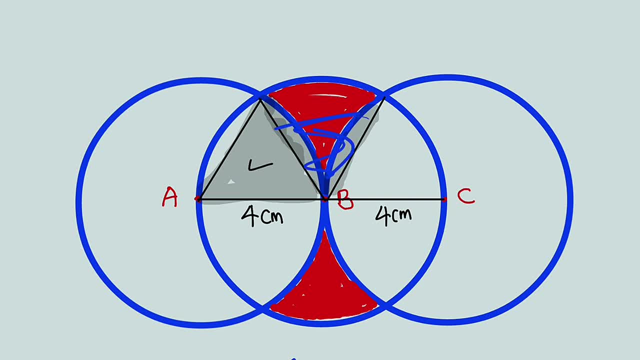 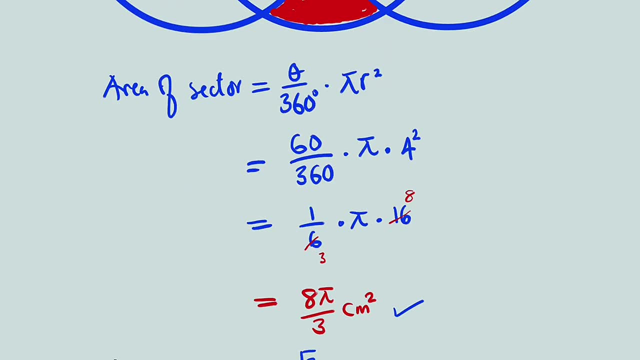 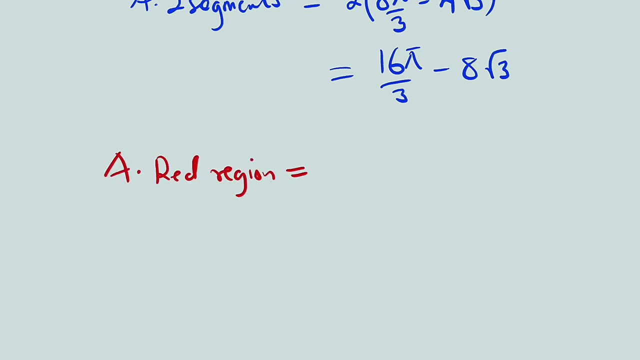 area of a sector Because entirely this is a sector. By subtracting the area of these two segments we end up having one area of this red region. So, area of red region, It's equal to the area of sector, minus the two area of the segments And the area of a sector. 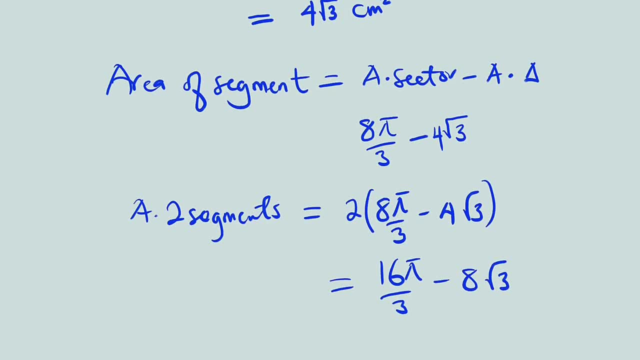 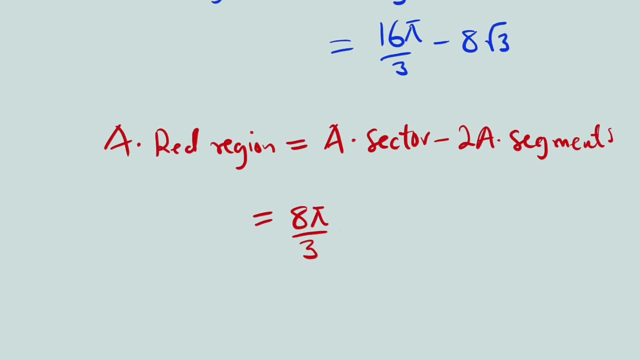 remain 8 pi over 30. So we have: this is equal to 8 pi over 30. Then we subtract this, The two area of segments, which is 16 pi over 30, they're minus 8 root 30.. All right, If you. 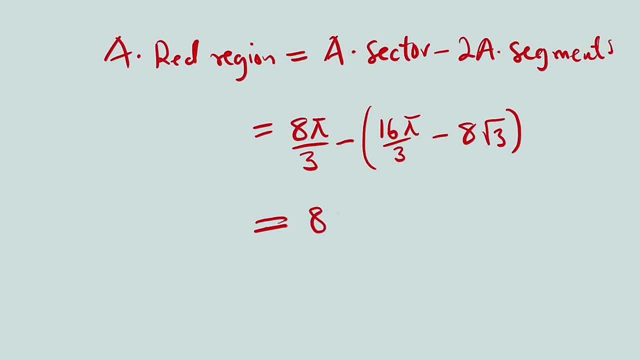 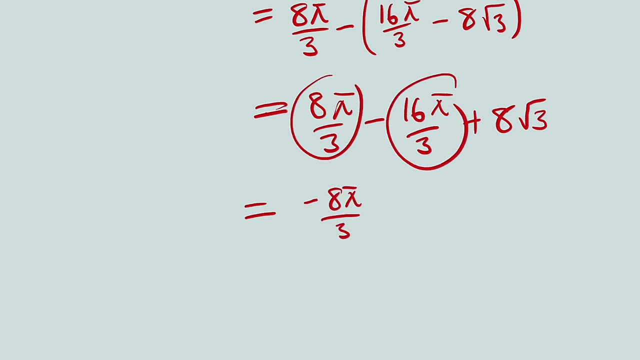 expand the bracket, we have 8 pi over 30 minus 16 pi over 30. Then plus because we are distributing negative sign inside. So from here we'll have negative 8 pi over 30. If you take away this from this, 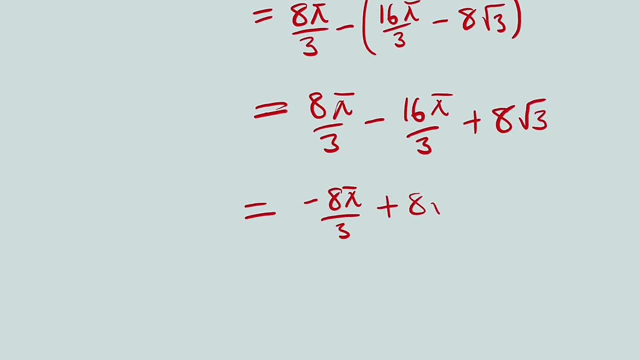 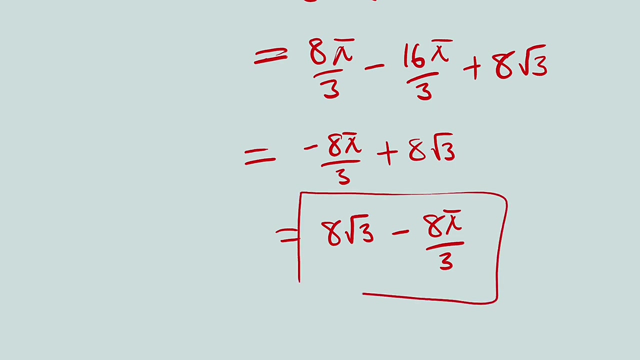 then plus 8 root 30, which we can rearrange as 8 root 30 minus 8 pi over 30. So this is the area of the red region. But remember we have two of them, We have one to the top. 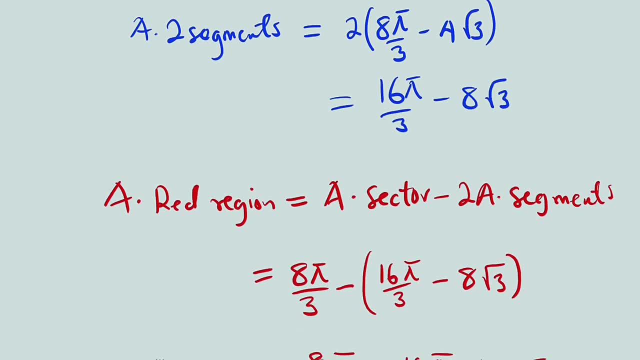 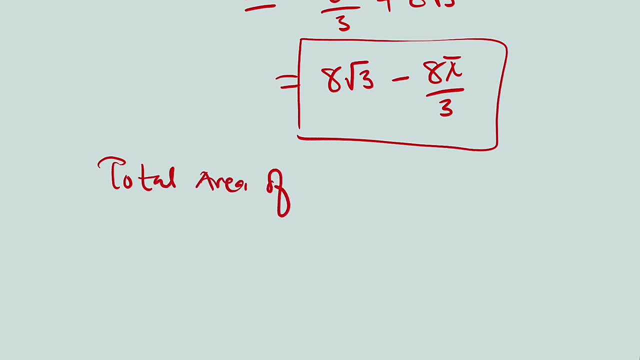 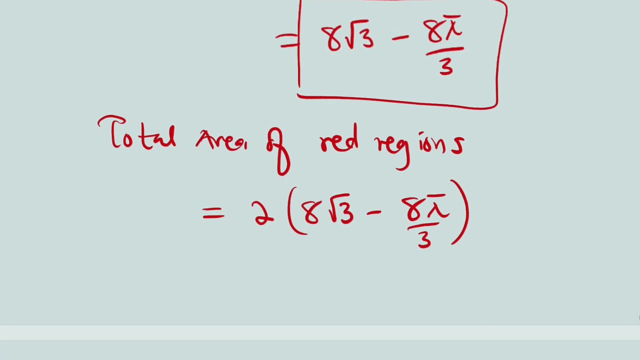 and one to the bottom. So all we have to do is to multiply this by two. So total area of red region is equal to 2 multiplied by 8 root 30, minus 8 pi over 30, which is equal to 16 root 30. 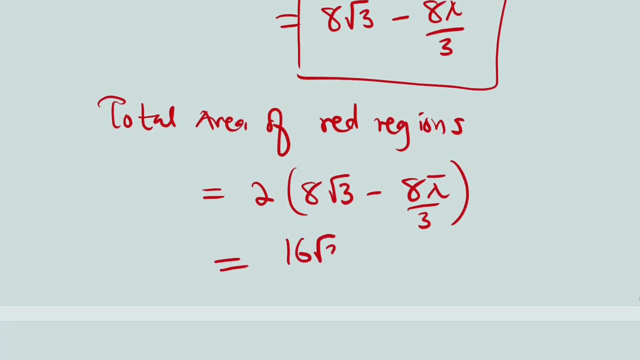 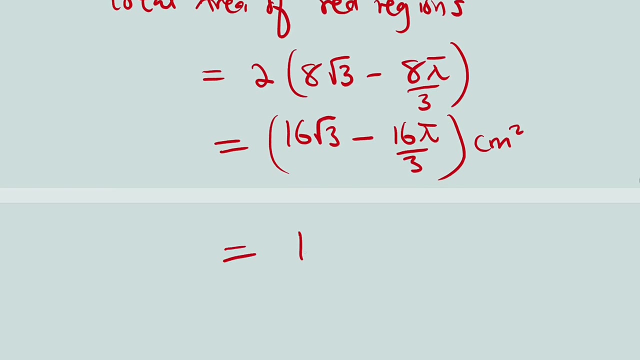 which is equal to 16 root 3 minus 16 pi over 3, all centimeter squared. if you like, you can factor out 16, which is going to give us 16 root 3 minus pi over 3 is all the same centimeter squared, and. 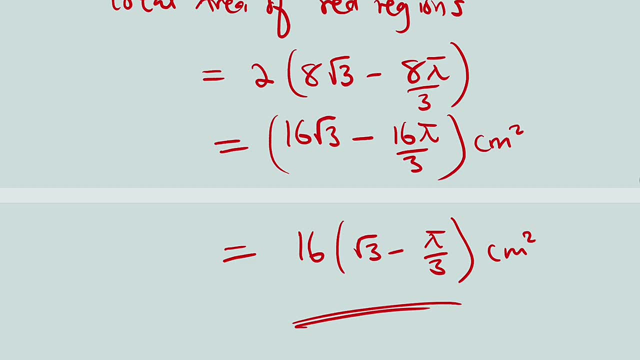 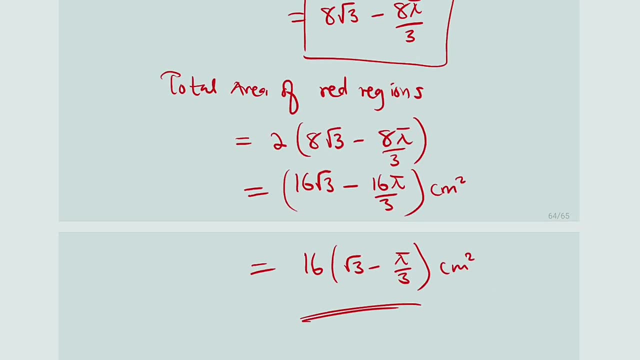 this is said to be the area of those two shaded regions, and this is all i have for you today. thank you for watching, do share to your learning colleagues and don't forget to subscribe to my youtube channel for more exciting videos. bye.